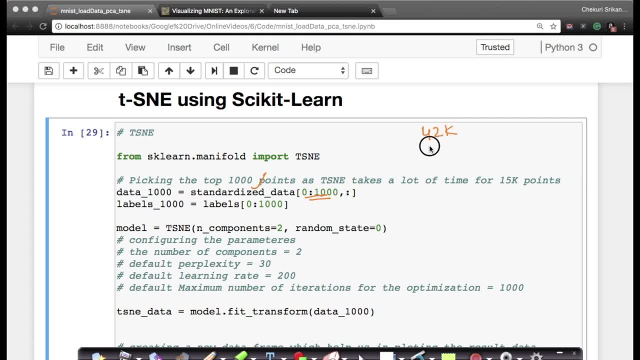 A point right in the actual data set. in standardized data I have 15K points. This new on 15K points takes about 10 to 15 minutes to run, depending on your laptop. Of course, on my laptop it takes about 20 minutes, OK. 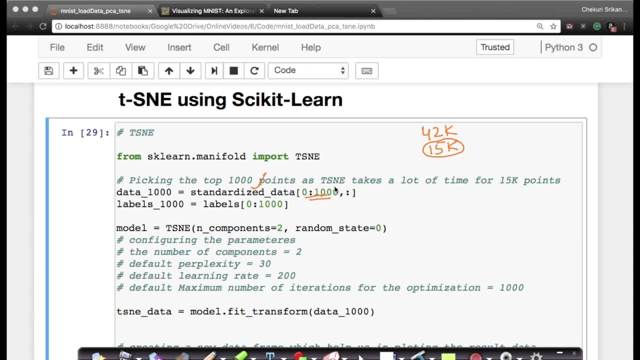 And so, just just for simplicity, I want to showcase, showcase. I want to show you the example with thousand points. So I'm just picking the first thousand points and putting it in a data set called data underscore thousand. Similarly, I'm taking the top thousand labels and I'm putting it as labels underscore thousand and I'll write the code with thousand. 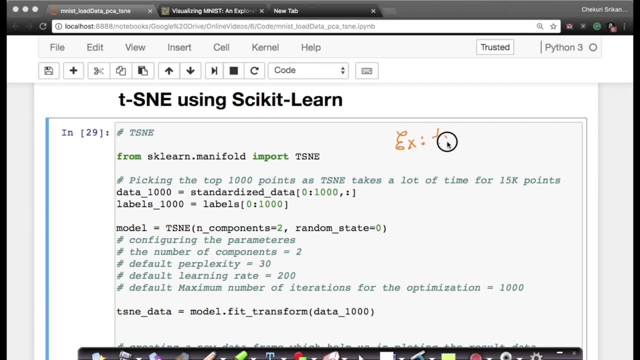 But remember, as an exercise, I strongly recommend you try T-SNE, you try T-SNE on 15K points and also on 42K points. OK, it will take you longer. You might have to. you might have to start running the code and take a coffee break or take a. take a stroll out. 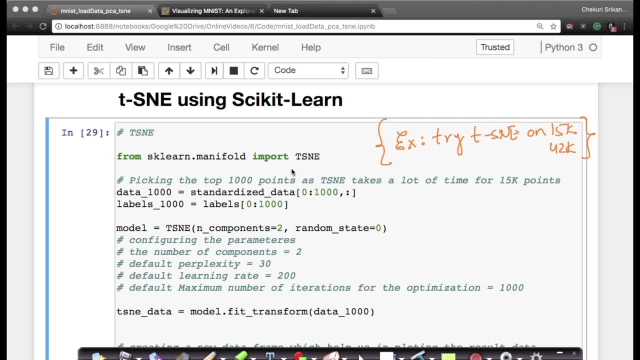 take a walk outside and then come back to find your results being there. OK, it takes. it takes a little longer Then than usual then you're typically used to in computer science. OK, so now let me define my model. My model can be defined very, very easily. 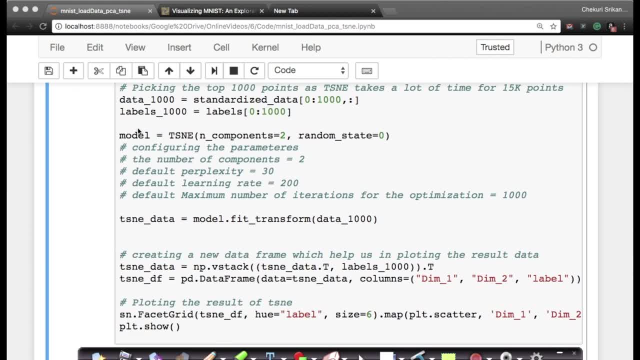 It's literally one line of code. OK, so I want my. I'm defining my T-SNE model, The variable is model and the function that I'm calling is the T-SNE constructor. And I'm saying my number of components is two and the random state is zero. 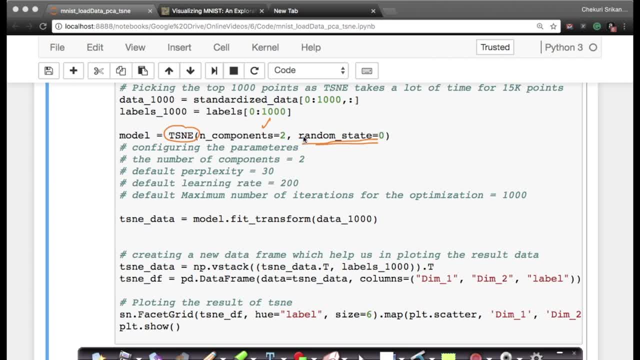 T-SNE is a randomized algorithm, which means if you don't define this, then if you run T-SNE two times you'll get slightly different results. by ensuring that the random state is always set to some number, You're going to get consistent or same results from one, from one run of this program to the second run. 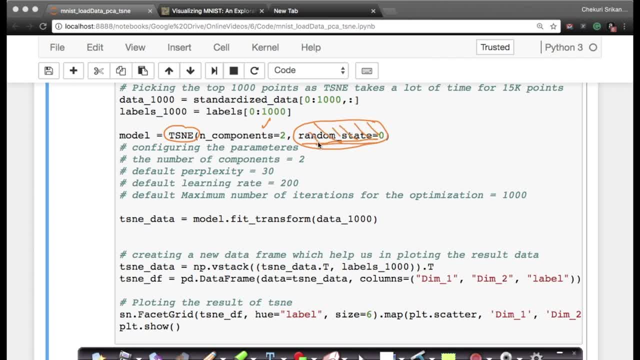 If you skip this, running T-SNE on the same data set two different times might result in slightly different outcomes. OK, because T-SNE is a randomized algorithm. OK, for those of you who don't know what randomized algorithms are: these are algorithms which will give slightly different results if you run them two or more times. 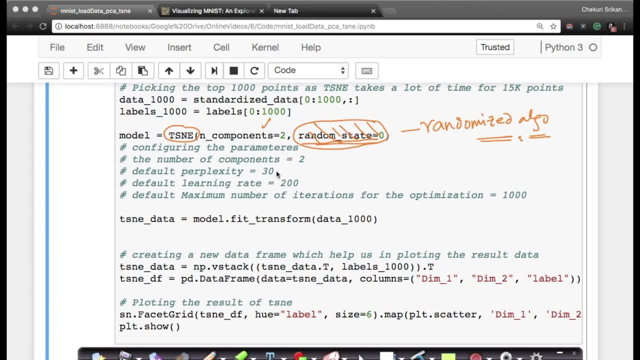 OK, now let's look at some default parameters. The default perplexity is set to 200 and learning rate is set to 200. So the default perplexity is set to 30.. OK, and the default maximum number of iterations is 1000 iterations. 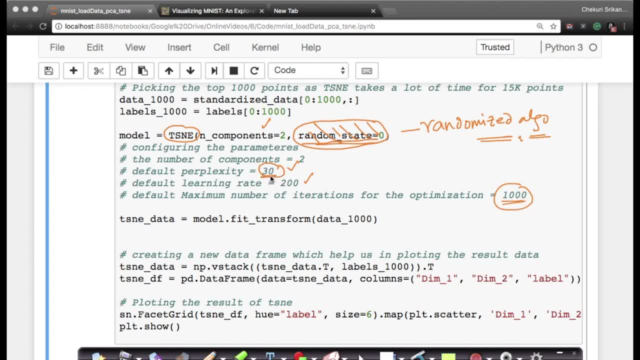 So I leave the values at 30 and 1000.. These are the two most important things that we will use. OK, this is your perplexity, as, as we have studied in the theory part, Perplexity is one of the most important parameters, along with number of iterations. 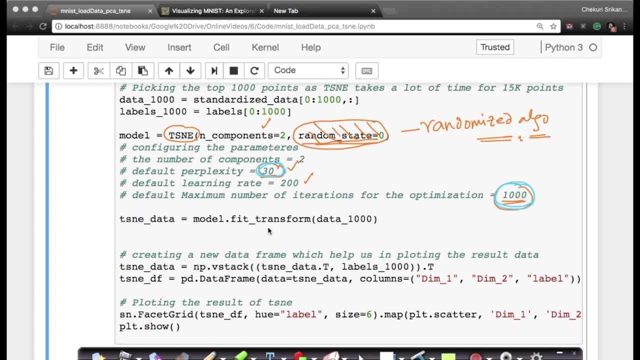 OK, so let's, let's just leave it at 30 and 1000 and I'll just say: model, dot, fit, transform, OK. this basically takes my thousand data points and creates T-SNE data, which is of course two dimensional. 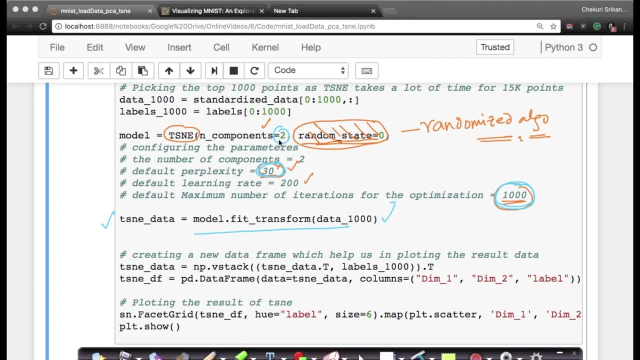 because I'm saying the number of components is two here Right now. what I'll do is the standard simple exercise. I basically combine my T-SNE data with label data. OK, I'm creating a new column called labels using NumPy's VStack or vertical stacking. 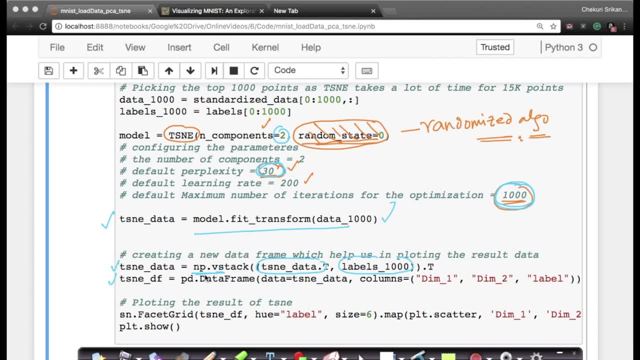 OK, and I'm converting this T-SNE data into a data frame with, with the first column being named dimensionality one, with the first column named dimensionality one, second column named dimensionality two, the third column being label. again coming from here, 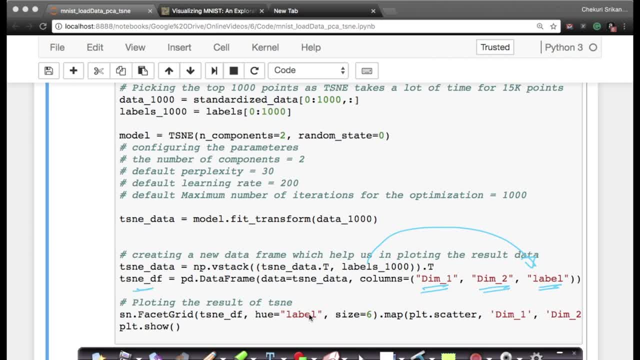 OK, once I have a data frame, I can now plot it using facet grid. OK again, with my hue as labels, with my coloring as labels. Well, let's go and see the plot that we have. The plot that we have looks like this, literally like this: 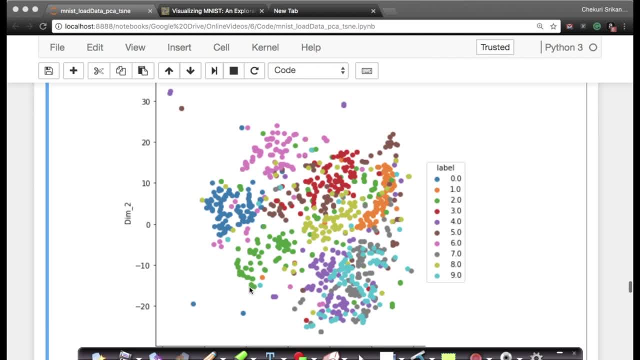 Now, let's see, This looks way better than our PCA. Now, if you look at this- and this is, by the way, this is just thousand points And with the perplexity of 30. And just thousand iterations, very, very simple. 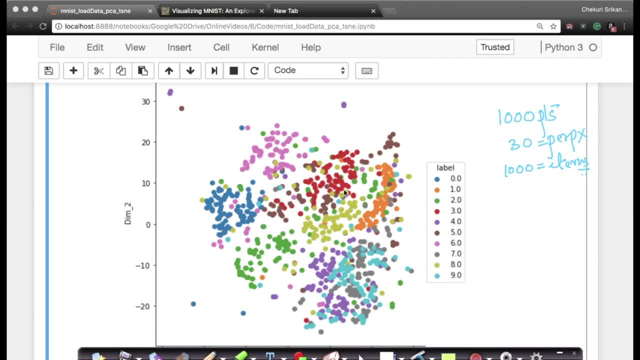 Remember, all of our PCA was on 15000 points. This makes very good sense. All of your zeros are well clustered here. All of your twos are somewhere in this region. Of course there are some small overlaps here and there. 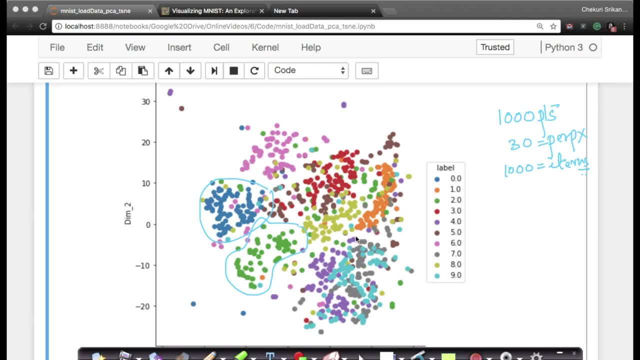 Your nine is more widely spread and things like that. And remember, this is just thousand points and a perplexity of 30.. If I just had 15000 points or all the 42000 points, And if I run it to 5000 iterations or even 10,000 iterations, this value could be much better. 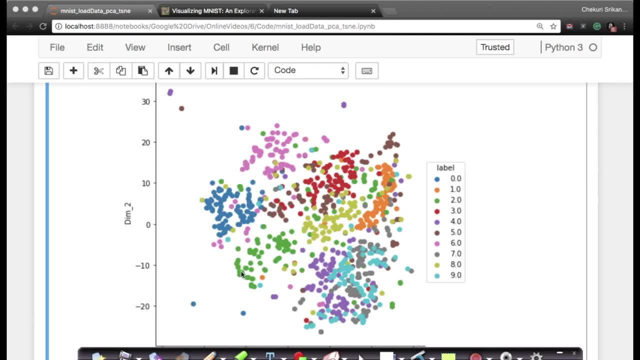 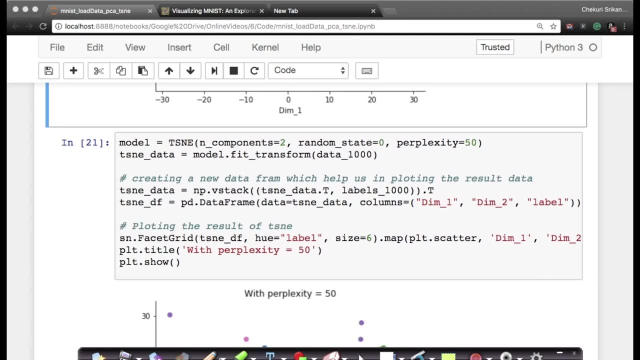 That's what I want you to explore as an exercise. I'll tell you I'll come to the exercise little later. OK, Now what if? what if I change the perplexity? OK, so in my code it just literally one parameter change I'm giving. 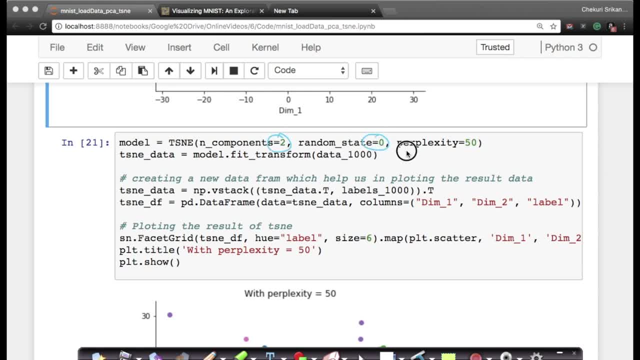 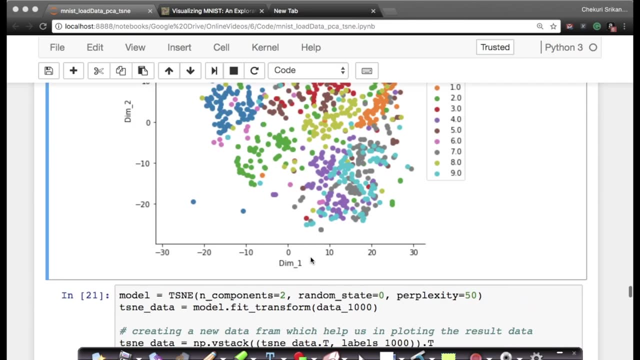 the number of components as 2, my random state as 0. I'm just changing my public state to 50, that's all. the rest of the code is exactly the way we saw earlier. okay, now, when I see this, this looks very much. this is perplexity 50. remember, this looks very much like my this code here with 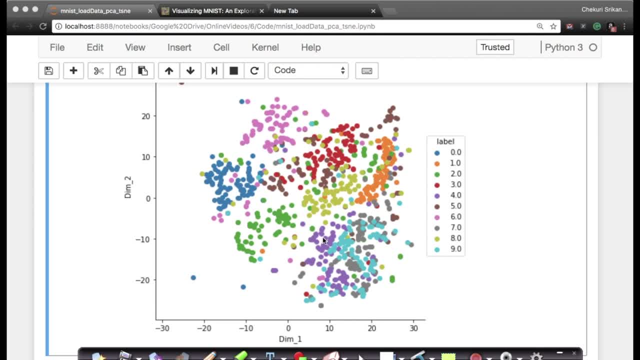 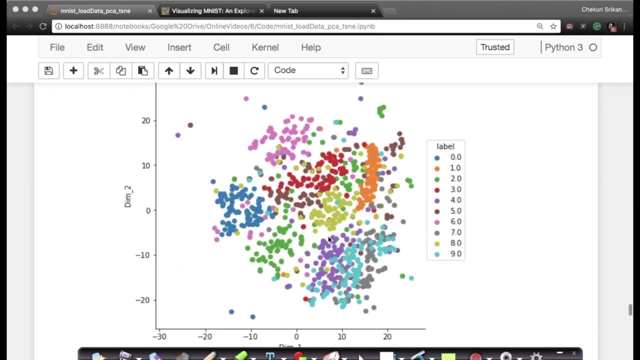 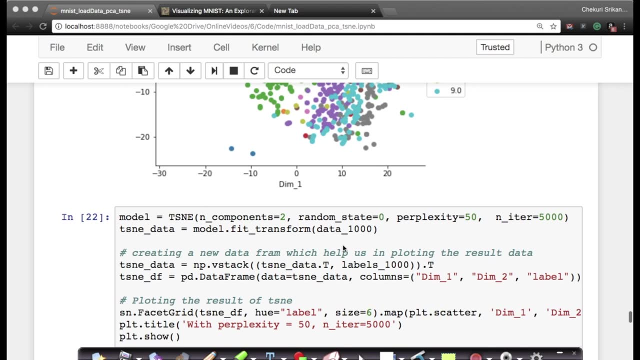 perplexity 30. that shows that, okay, around 30 or 50 perplexity seems to make sense for 1000 points with 1000 iterations. right, this looks very, very similar, almost almost identical, with probably small variations. okay, now the next question here is what if I increase the number of iterations? 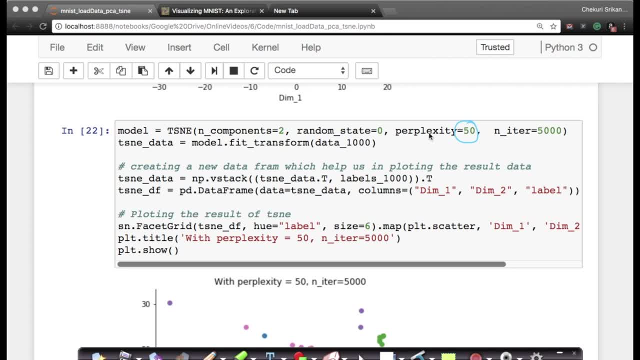 okay. so perplexity: 50 seems to be fairly stable and 30 to 50 seems reasonably stable. and my random state: I'm just setting it to 0. now, instead of 1000 iterations I want to make the number of iterations equals to 5000. rest of the code stays the same. okay, now when I go from 1000 iterations. 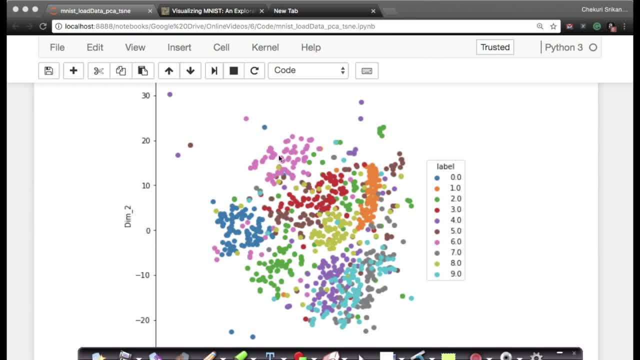 to 5000 iterations, the shape is very, very stable. these are the lessons that we learned in distalpub right that we need to. we need to try various values of perplexity. so we tried 30 and 50, this, this and with with 1000 iterations, and both the shapes looked fairly stable. then we increase the number. 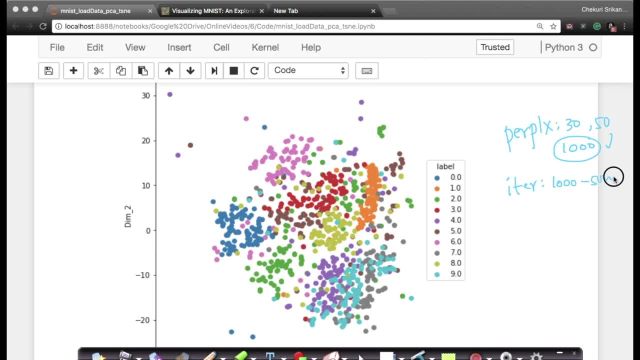 of iterations from 1000 to 5000, and the shape still remains fairly stable. okay, so we can take this 4000 points, of course, 4000 points. this shape seems to make pretty good sense, of course, remember, when you go from 1000 points to 15000 points, or 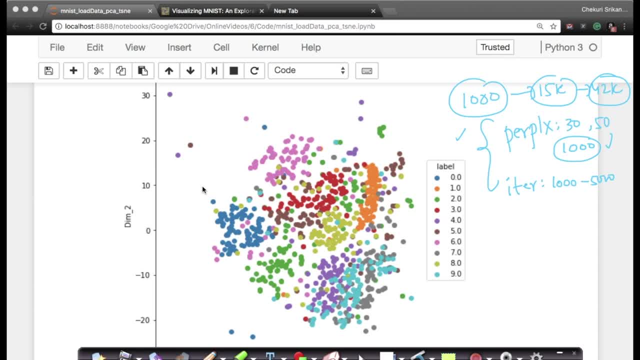 even for 2000 points, the shape, the points will be much well separated because that's more information out there. there is more information which makes so my. the ideal outcome here is if you take 42k data points and you try various perplexities around 30, 50, etc. find the good perplexity and 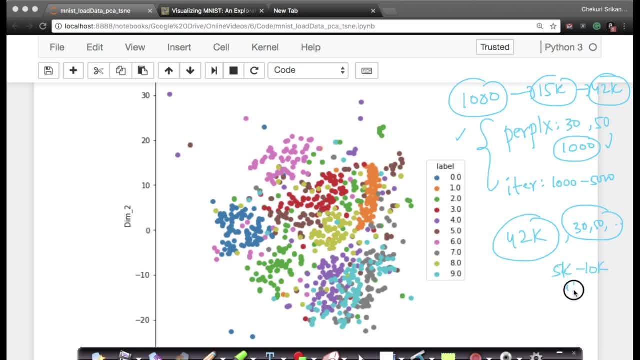 run up to 5k to 10k iterations. okay, that, that that's what I'm trying to say here. so that's what? that? that, that that's what I think will give you one of the best results out here. again, that's something for you to explore, that's an exercise that I leave it for you to explore and understand.